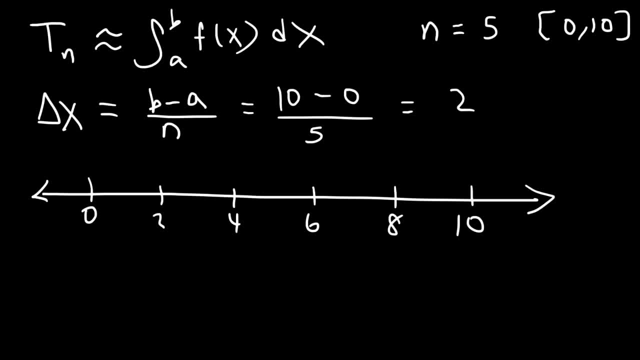 And delta x is going to be 2.. Now, I don't know if you saw an earlier video that I created on Riemann sums- left endpoints, right endpoints- and another video on midpoint rule, But if you watch those then you know my methods when it comes to using a number line for these kinds of problems. 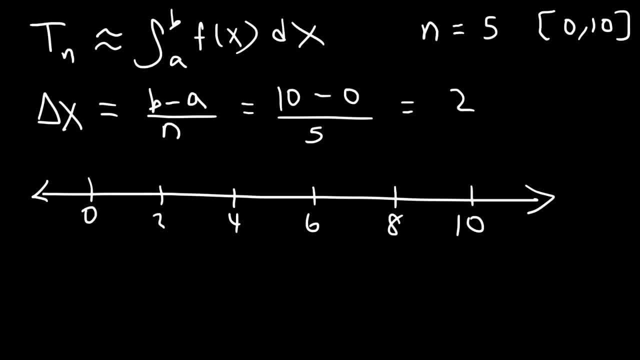 Now just to recap: using the left endpoint for a Riemann sums problem, you would have to choose 5.. 5 points out of the 6 points listed, since n is equal to 5.. There's 5 intervals and you would have to choose 5 of the 6 points. 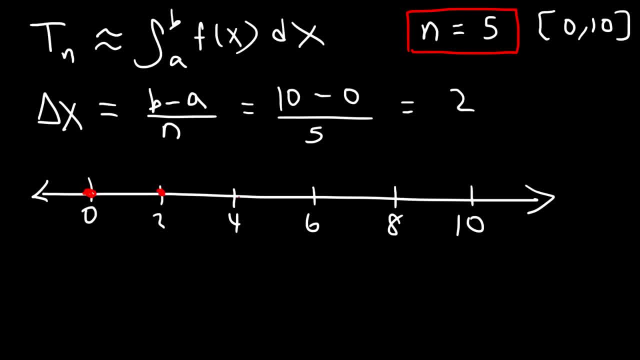 So the left endpoint rule, you would use 0,, 2,, 4,, 6, and 8.. Now, if you wish to do a Riemann sums problem using the right endpoints, you'd have to use these 5 out of the 6 endpoints. 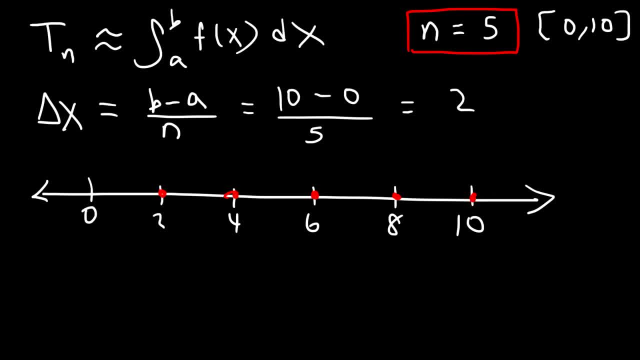 So one of the endpoints you won't be using, I mean one of the points. They're not all endpoints, So you're always going to use 5 out of 6 points if you're using the left endpoint rule or the right endpoint rule or the midpoint rule. 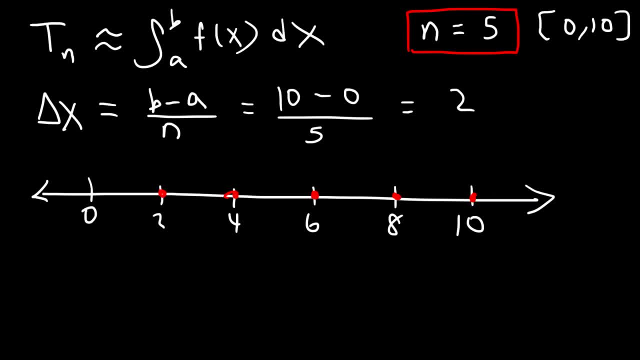 So, using the right endpoints, it's going to be 2,, 4,, 6,, 8,, 10.. And now, if you're employing the midpoint rule, you would simply pick the points in the middle, like 1,, 3,, 5,, 7, and 9.. 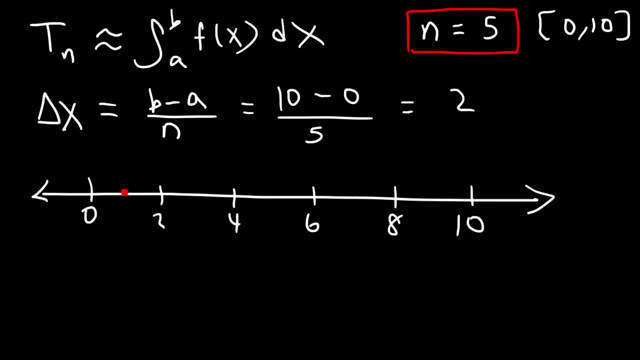 For the trapezoidal rule, you should use all the points in the middle. You're not going to use 5 out of the 6 points, You're going to use all of them, And so that's how the trapezoidal rule differs in one way from using the left endpoint, the right endpoint or the midpoint rule. 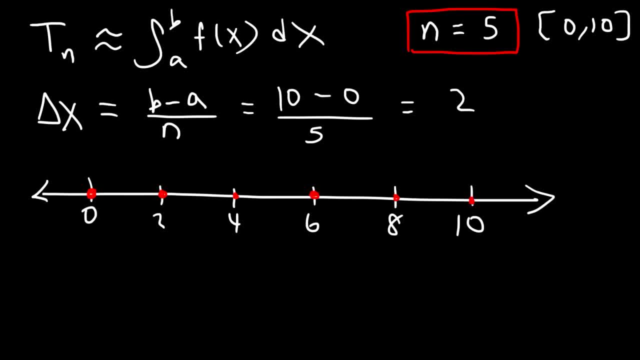 Now what is the formula for the trapezoidal rule? The area of the rectangles will be equal to delta x divided by 2.. These are the sum of the area of the rectangles. The area of the rectangles times f of x 0, plus 2 times f of x 1, plus 2 times f of x 2.. 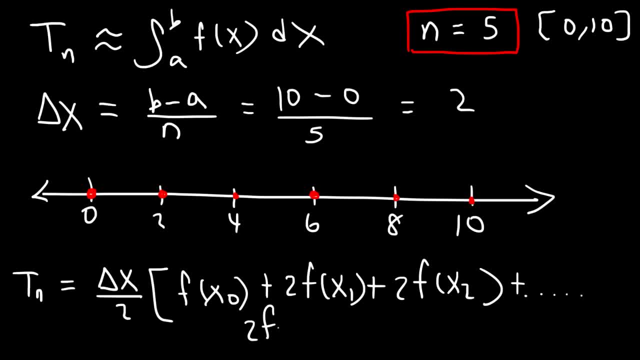 And then it's going to continue. The second to last one will be 2 f of x n minus 1.. And the last one will be just f of x- n. So here's what you need to know for the trapezoidal rule. 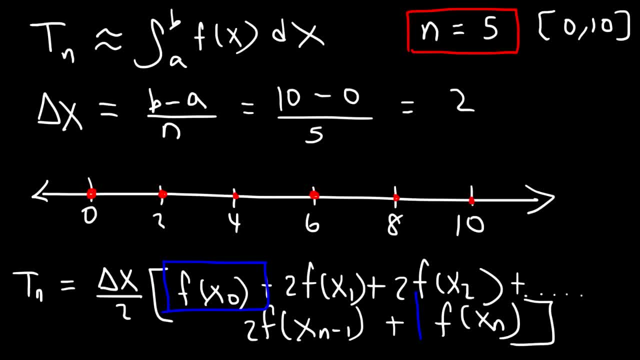 1., 2., 1. And the last one. these are y values. do not multiply those by 2.. All of the y values in the middle. multiply those by 2. And 2 times 1 half will give you 1.. 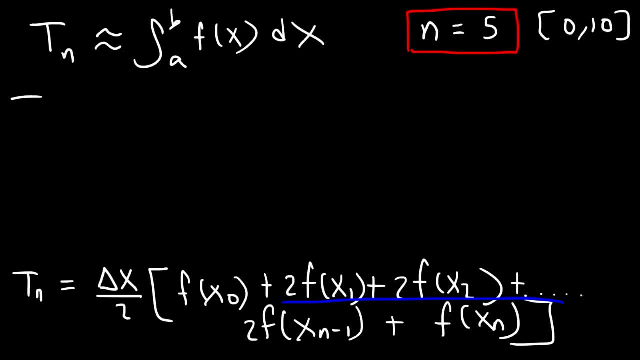 Now let's finish this example. So t sub n, where n is 5, we're going to have t sub 5. That's equal to delta x over 2.. And this example, delta x we said was 2.. 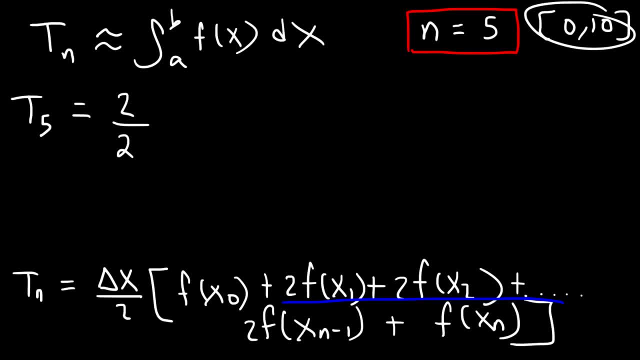 It was 10 minus 0 divided by 5.. Now what's x0 and x1?? Those are the points that we had on the number line. The first x value was 0, and then it went up by 2s because delta x is 2.. 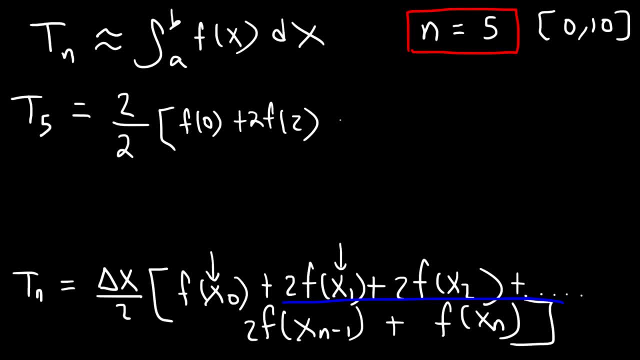 So the next one is going to be f of 2,, but we need to multiply that by 2.. And then 2 times f of 4,, plus 2 times f of 6, and 2 times f of 8.. 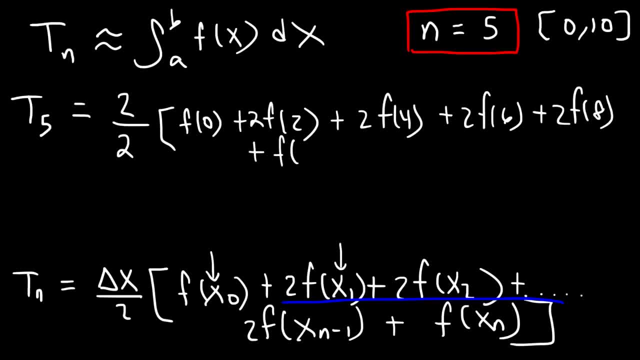 1. And the very last one. we're not going to multiply by 2.. So f of 10 is the last one. So keep that in mind, The first and the last one. do not multiply that by 2.. So never multiply these two y values by 2.. 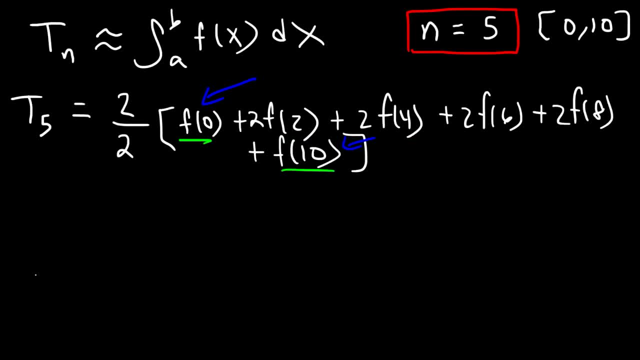 But the middle ones. you need to do so. So 2 divided by 2 is 1.. And keep in mind: f of x is x squared in this problem. So f of 0, that's going to be 0 squared, so that's 0.. 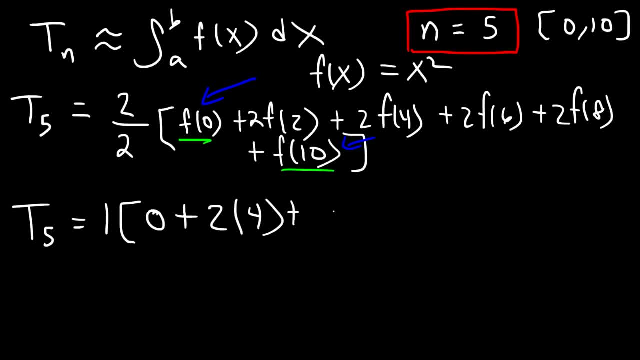 And then f of 2,: 2 squared is 4,, 4 squared is 16,, 6 squared is 36,, 8 squared is 64, and 10 squared is 100.. And don't multiply that by 2.. 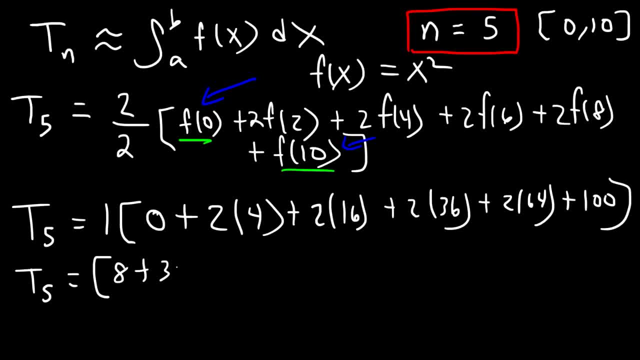 Now, 2 times 4 is 8.. 2 times 16 is 32.. 2 times 36 is 72.. 2 times 64 is 128, and then plus 100.. Now 8 plus 32, that's 40.. 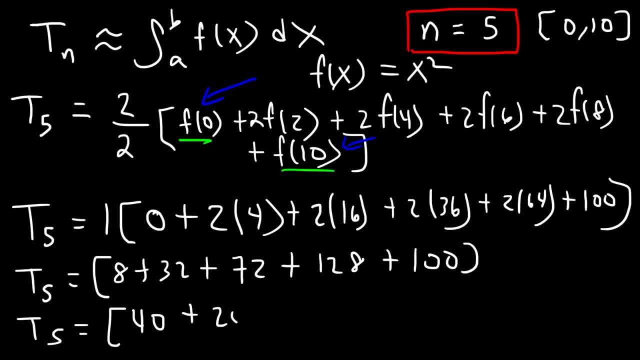 72 plus 128, that's 200.. And 200 plus 100 is 300, plus 40. This will give us 340.. So that's the approximate area under the curve. So now let's calculate the exact answer. 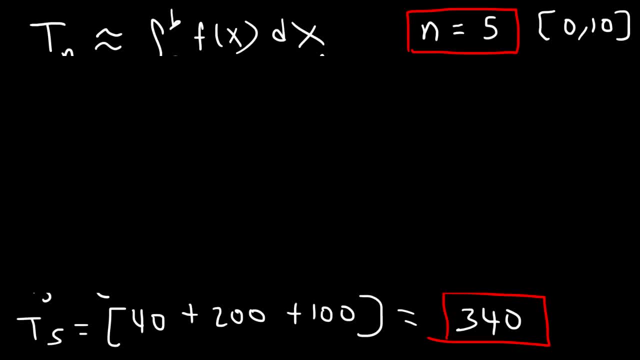 So the exact answer is going to be the integral from a to b, 0 to 10, x squared dx. So the exact answer is going to be the integral from a to b, 0 to 10, x squared dx. The antiderivative of x squared is x cubed divided by 3, evaluated from 0 to 10.. 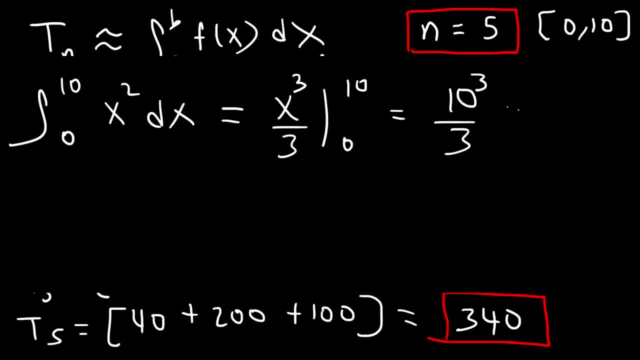 So if we plug in 10, it's going to be 10 to the 3rd over 3.. And then if we plug in 0, that's just going to be 0.. 10 times 10 times 10 is 1000.. 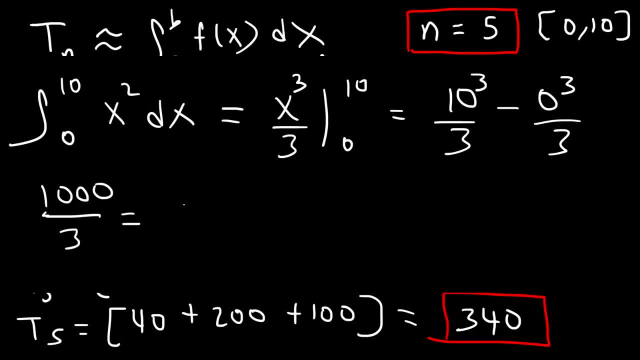 10 times 10 times 10 is 1000. So we have 1000 divided by 3.. So the exact answer is 333.3 repeated, And so this represents the area under the curve. As we see in this example, the trapezoidal rule did a very good job in approximating. 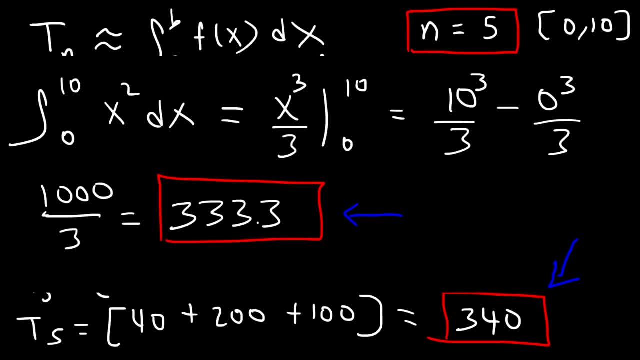 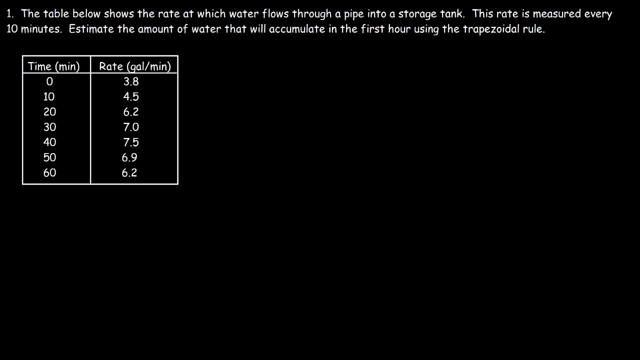 the exact answer of the area under the curve 340 is very close to 333.3. And so the trapezoidal rule is a very good approximation If you wish to evaluate the definite integral or find the area under the curve. 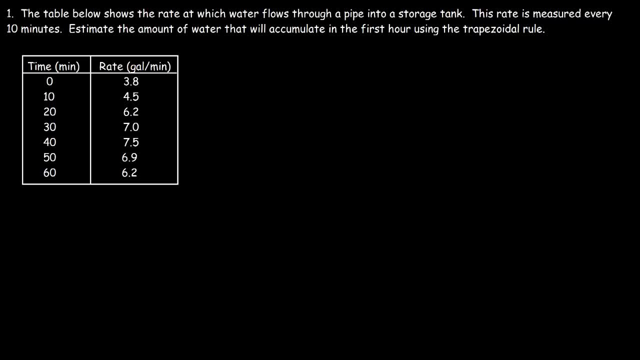 Let's work on this word problem. The table below shows the rate at which water flows through a pipe into a storage tank. This rate is measured every 10 minutes. Estimate the amount of water that will accumulate in the first hour using the trapezoidal rule. 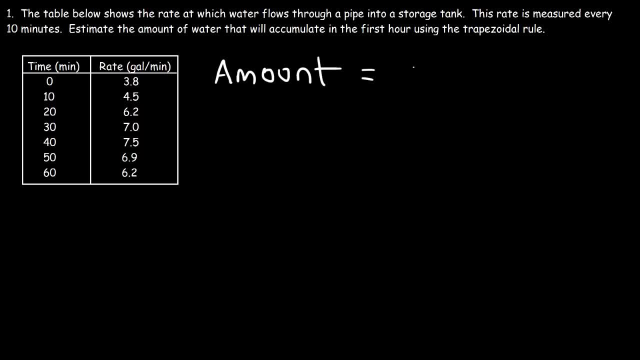 So we have one of those accumulation problems. The amount that will be accumulated is equal to the definite integral of the water flow rate as a function of t- dt. Now we don't have a function for our t, So we have to estimate this value using the trapezoidal rule. 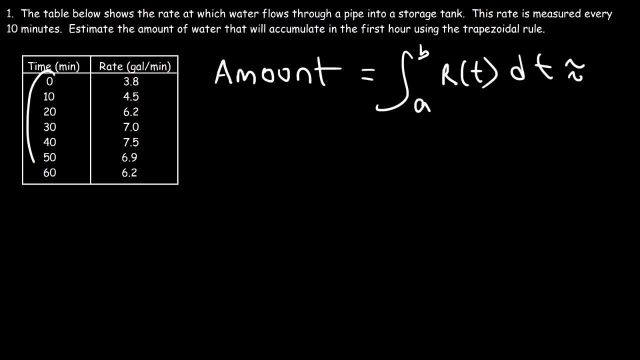 And we have a total of seven points And so we have six intervals. So this is gonna be t sub six, So n is six in this example, On the interval zero to 60.. So if we calculate delta x, it's gonna be b minus a divided by n. 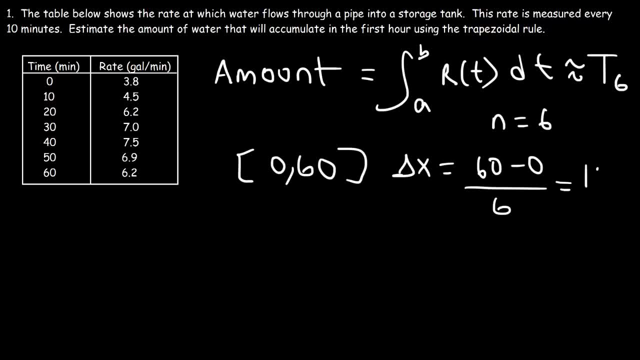 So that's 60 minus zero divided by six, And so we can see that delta x is 10 minutes. So now, using the trapezoidal rule, it's gonna be delta x divided by two times the first point, f of zero, and then plus two times f of 10. 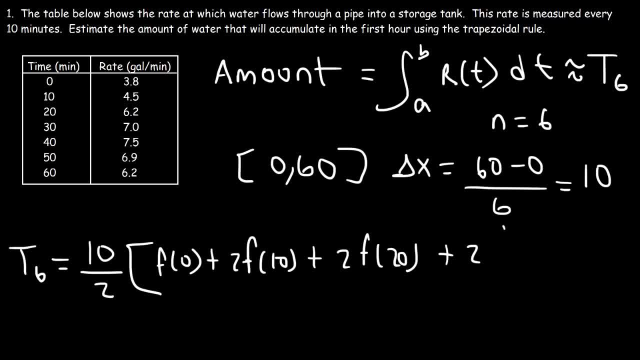 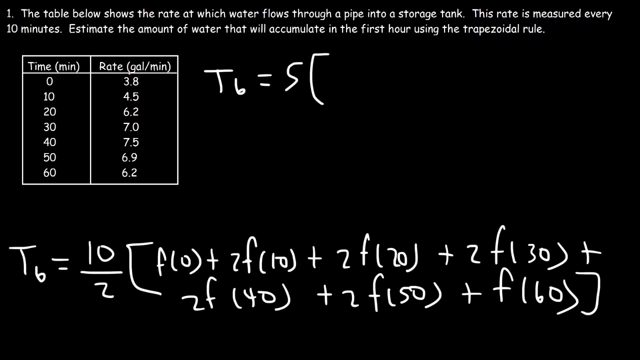 plus two times f of 20, all the way to f of 50.. And the last one: we're not gonna multiply it by two, It's just gonna be f of 60.. 10 divided by two is five. F of zero based on a table. 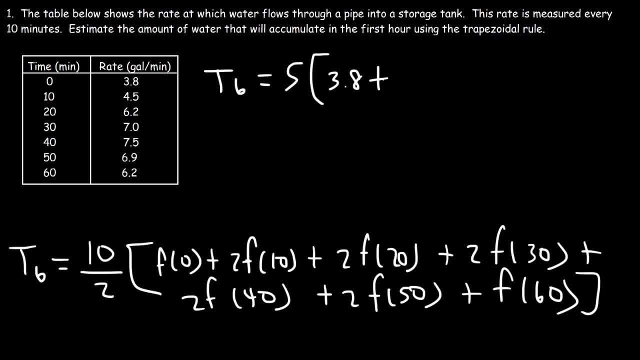 it's 3.8 gallons per minute. Now if you multiply the minutes- because it was 10 minutes- divided by two times the gallons per minute, you're gonna get the amount of water that accumulates into the tank in the unit of gallons. 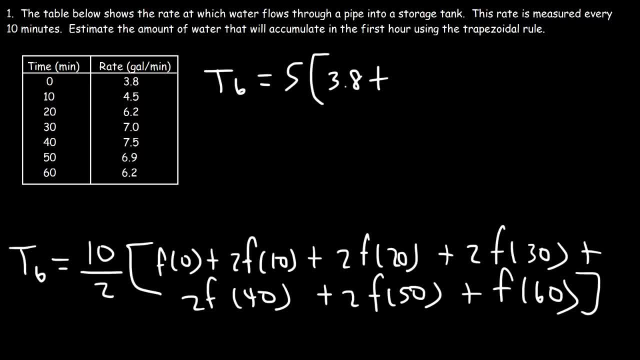 Now this is gonna be two times f of 10.. So at 10, the rate is 4.5.. And then, for f of 20,, the rate is 6.2. And then at 30,, the rate is seven. 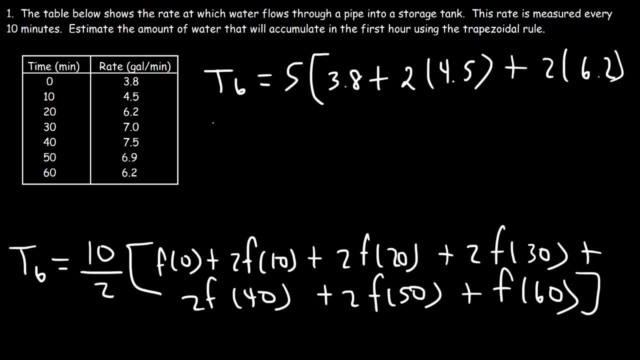 And at 40, the rate is 7.5.. At 50, it's 6.9.. And then at 60, it's simply 6.2.. But we're not gonna multiply that by two, So we're gonna multiply that by two. 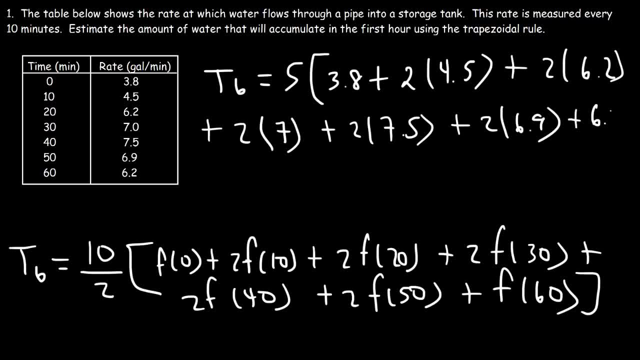 And then at 50, it's 6.9.. And then at 60, it's simply 6.2.. But we're not gonna multiply that by two. But we're not gonna multiply that by two. Now, two times 4.5 is nine. 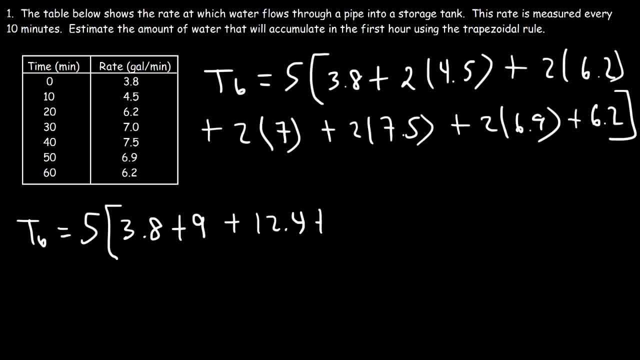 Two times 6.2 is 12.4.. Two times seven is 14.. Two times 7.5 is 15.. Two times 6.9, that's gonna be 13.8.. And then plus 6.2.. 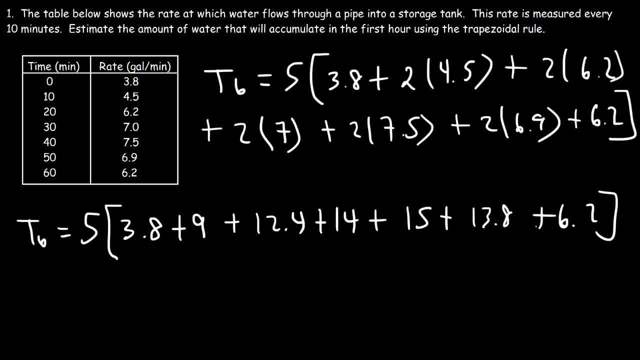 So you can type this into a calculator if you want to. So you can type this into a calculator if you want to, And this will give you 371.. And this will give you 371.. And the unit will be in gallons. And the unit will be in gallons. 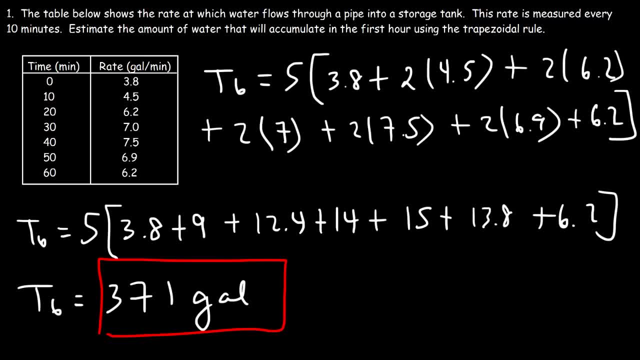 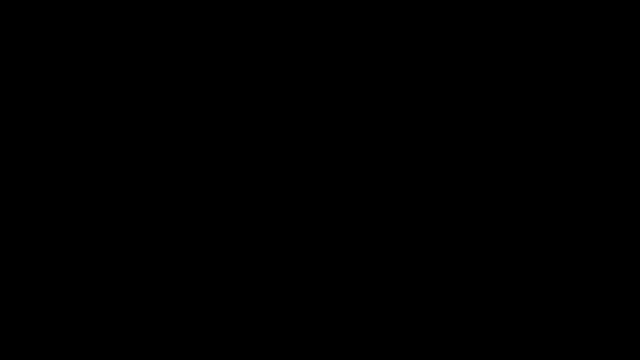 The exact answer might be different from this one, but it's gonna be close to it, Thank you. 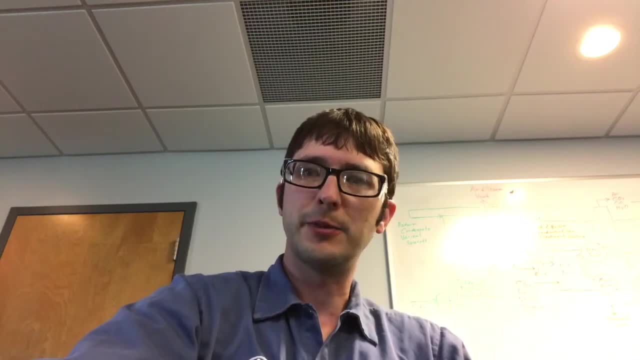 Hey folks, Brad Sutliff here for another chemical engineering concept video. Today we're going to talk about steam boiler systems, process flow diagrams and material balances. In addition to that, we're going to take a walk out in the field and see what. 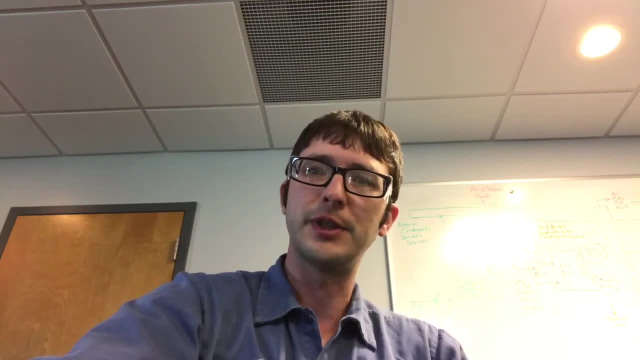 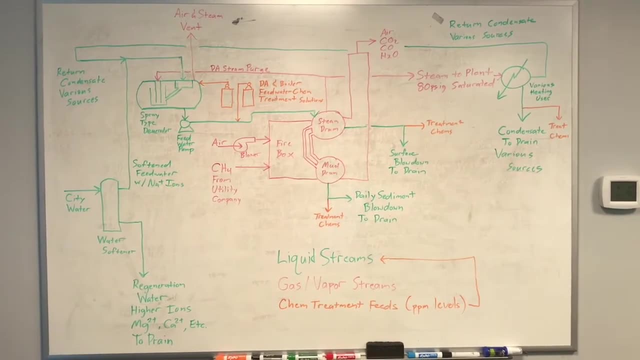 all this stuff looks like in real life for our small batch processing facility here in Lock Haven, Pennsylvania. Let's start with the process flow diagram for the boiler system which I have drawn up here on the whiteboard in our conference room. It all starts with the feed water. We basically